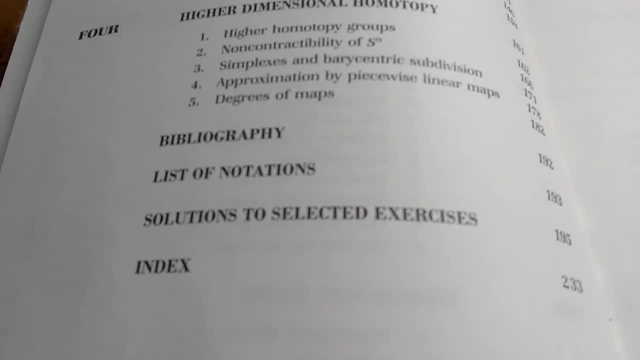 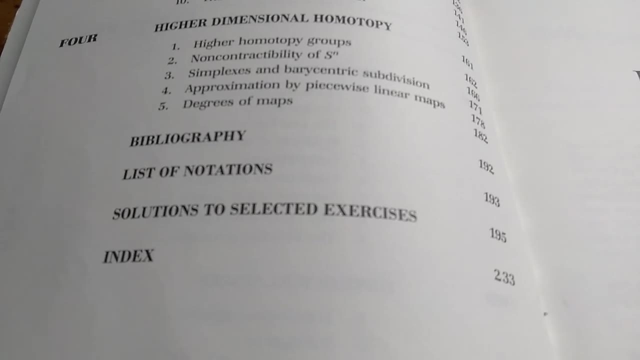 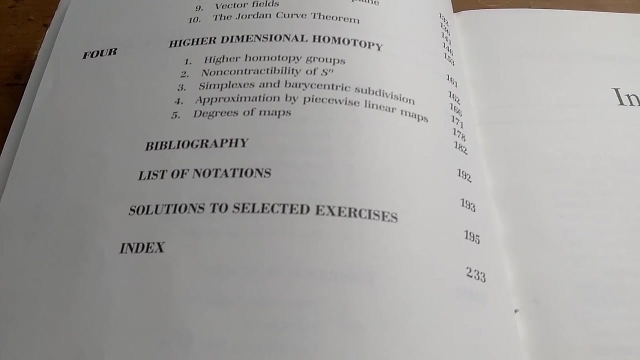 Notice it says Solutions to Selected Exercises. I think it has answers to all of the exercises, or at least most of them, So even the proofs, So it'll give you hints or key things worth mentioning regarding the proofs. That's a big plus if you're using this to self-learn. 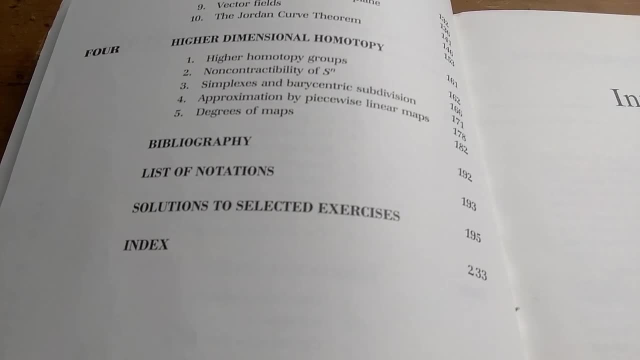 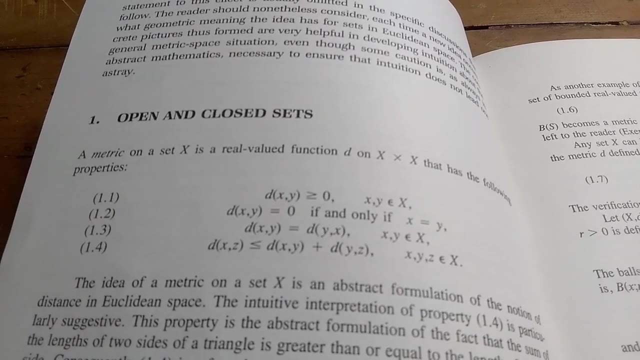 We'll look at some of the solutions in a minute and then compare The solutions to the actual problems. Let's take a look inside the book. Okay, so the readability of this book is excellent. It reads really well. It's written very well. 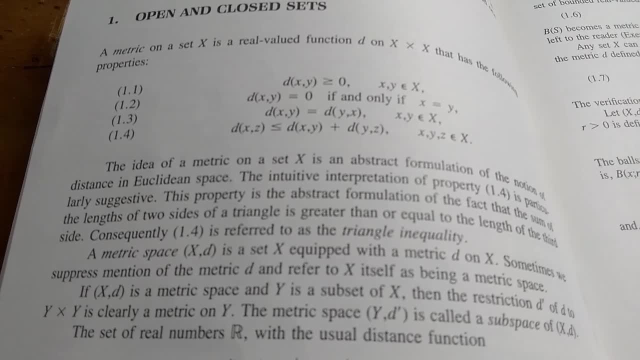 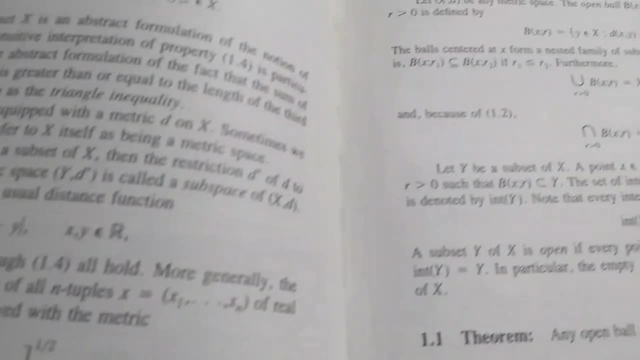 It's a really, really solid book. I would say it's not okay. I would say it's good or great. It's a really good book on topology, which is a really hard subject for people to learn on their own. Now a word of warning. 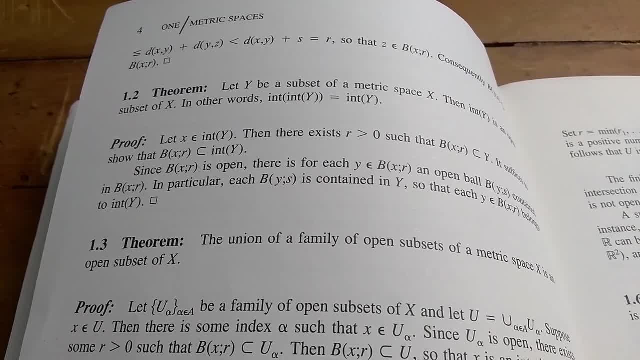 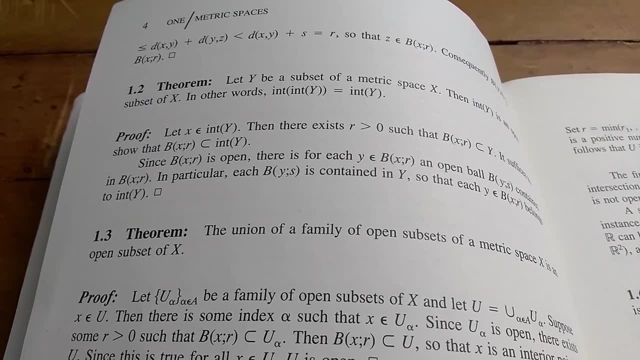 When you read this book, you should read it like you read a book, every other higher level math book, right? you sit down with a piece of paper and you know you read the theorem and you try to prove it on your own. and if you can't do the proof on your own, then you look at their proof and try to see what. 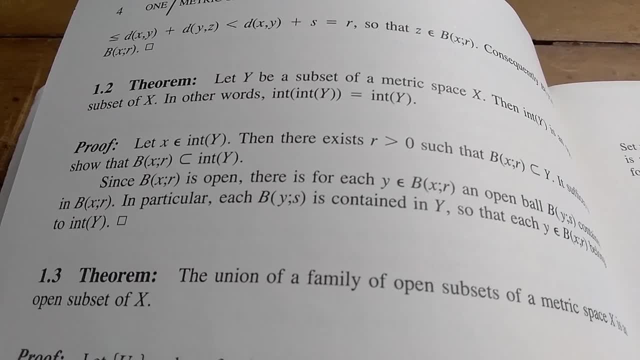 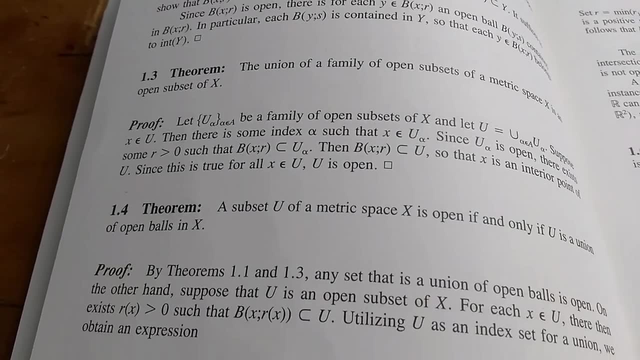 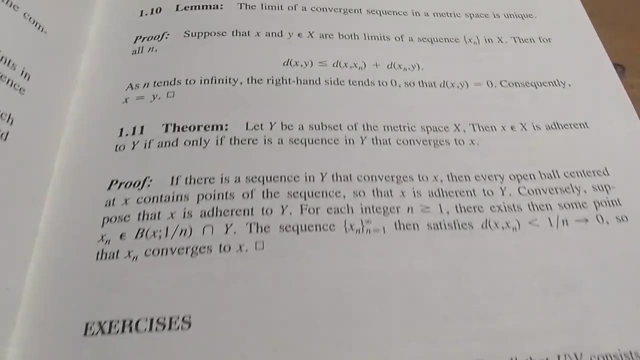 you're missing and then, once you find what you're missing, you go back and then you complete your proof. that's the best way to learn higher level math, right? always try to do stuff on your own. let's take a look at the exercises. okay, so these are the exercises for the first section, right? so let's see we have one. 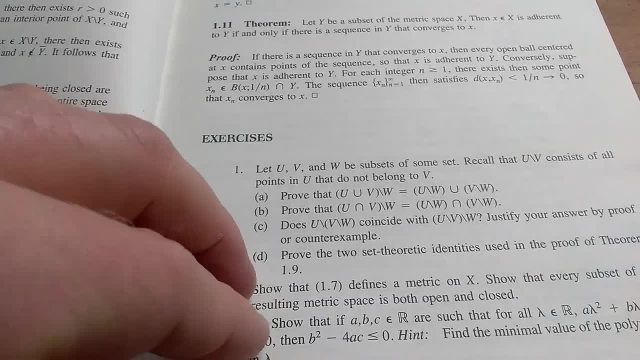 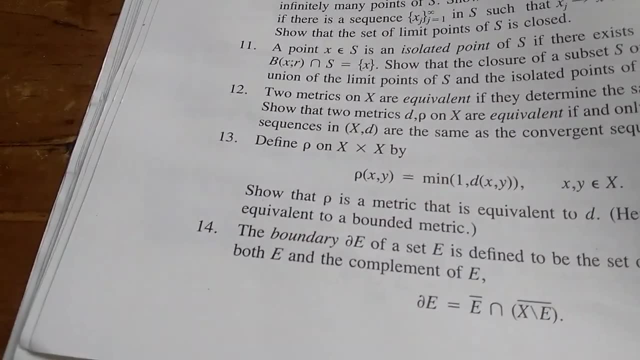 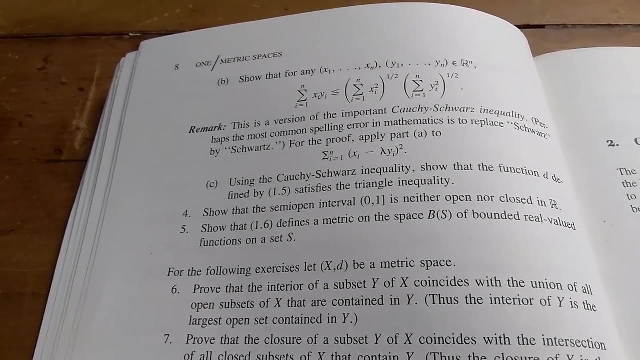 two, three, three problems so far, then we have four, five, six, seven, eight, nine, ten, eleven, twelve, thirteen, fourteen. so there are 14 problems in the very first section. now let's go to the answers to see how many of these problems we have answers for. these are the answers. that looks like a full proof. oh my god, wow so. 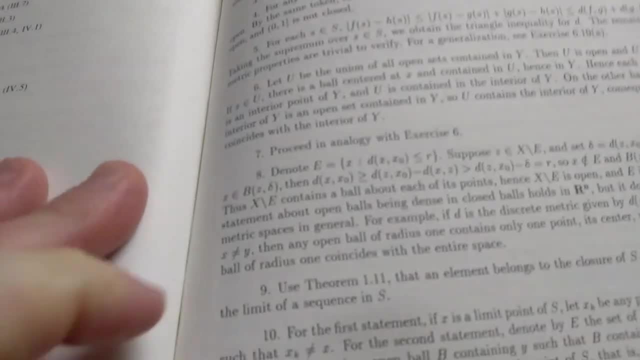 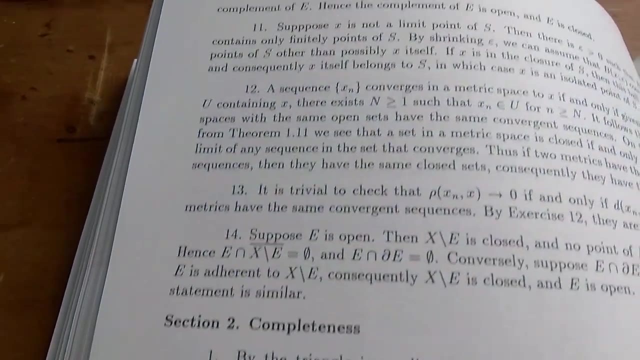 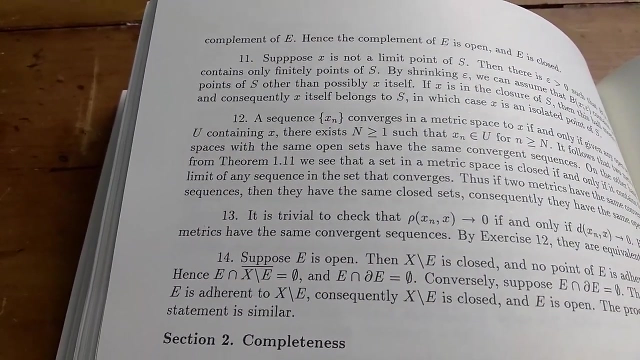 we have one, two, three, four, five, six, seven, eight, nine, ten- let's turn the page- eleven, twelve, thirteen, fourteen, yeah, so he goes through and answers every single one. now, these are probably not complete proofs- I'm sure they're not- but they're hints, so it's. 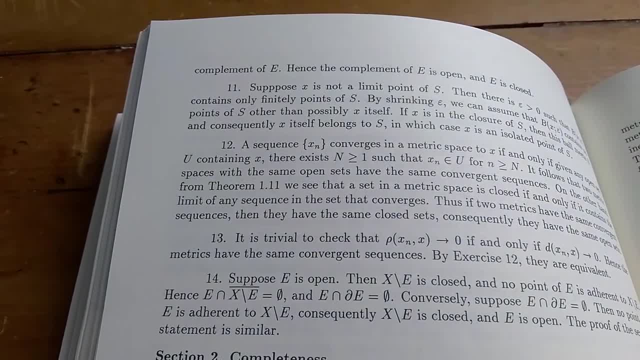 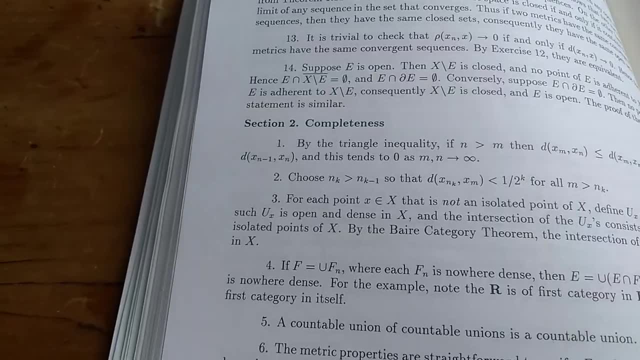 really, really nice to have this so you can try to do the proofs on your own, and then you can look in the back of the book and you can get the answers, or at least things that are missing. look at this: section two: one, two, three, four, five. 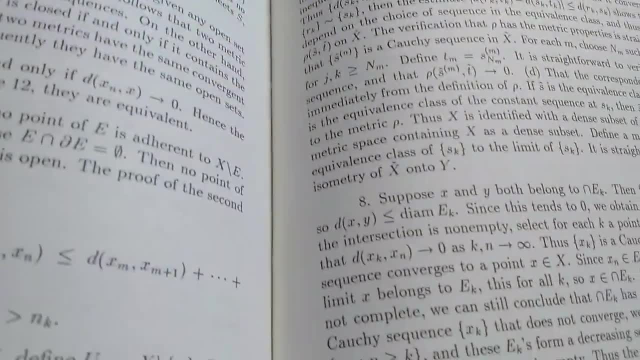 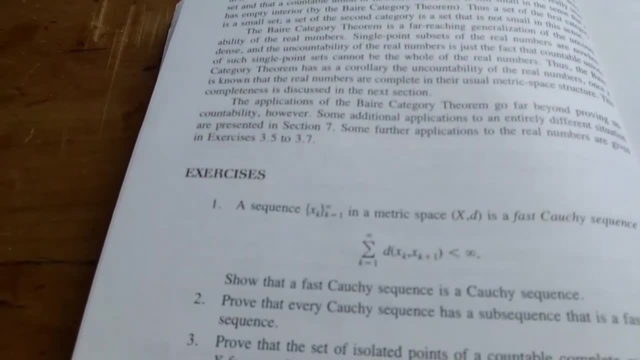 six, seven, and then he goes on to problem eight. so one through eight. let's go ahead and look in section two and see if there's eight problems. so this is section two and, as you can see, we have one, two, three, four, five, six, seven, eight. we have eight. 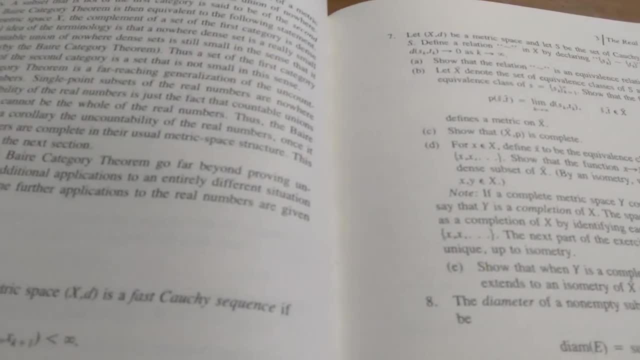 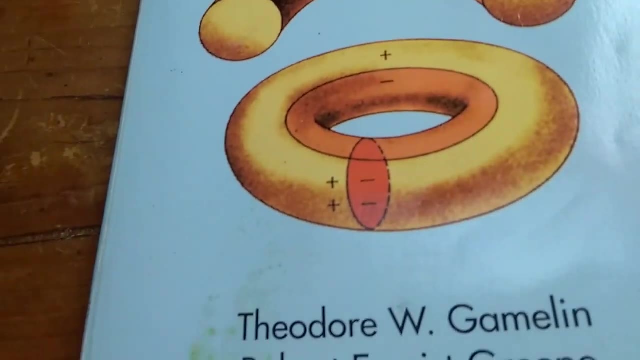 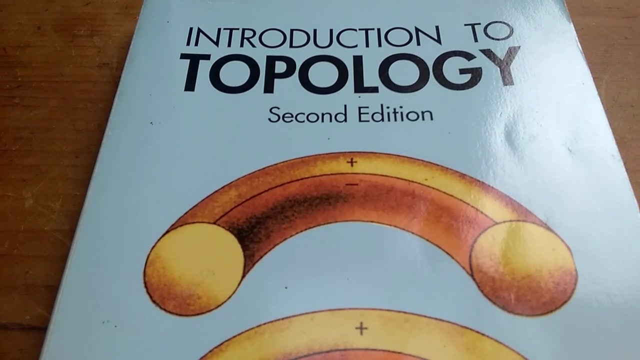 problems in section two. so yeah, he answers all of the questions for you. so again, the book is introduction to topology and the authors are gamelin and green. I use this as a supplement, not to learn topology on my own, but just as a supplement and as a reference book. it's actually really good. 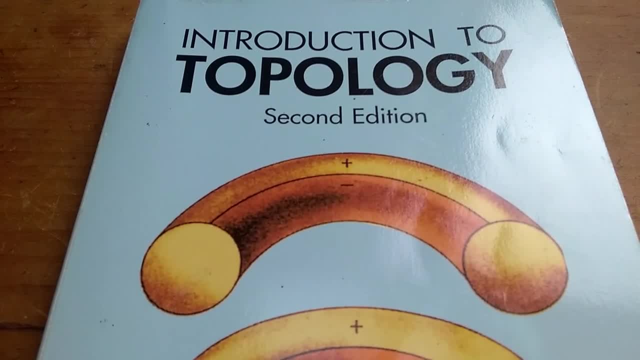 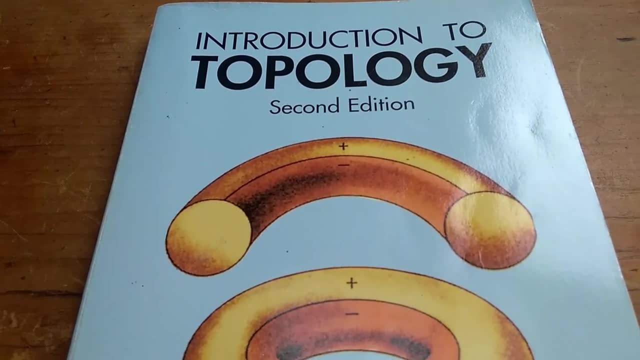 as a reference to. so I already knew a lot of topology before I read this book, so keep that in mind when you're reading the book. I hope this video has been helpful. 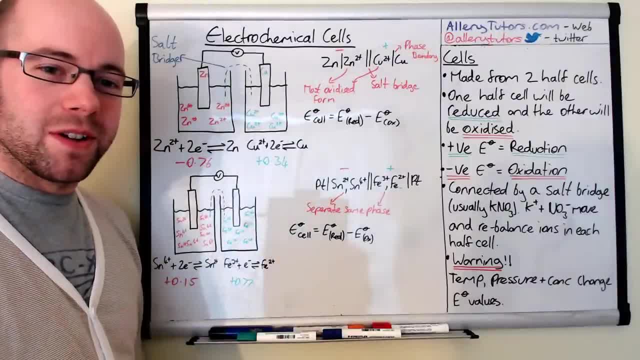 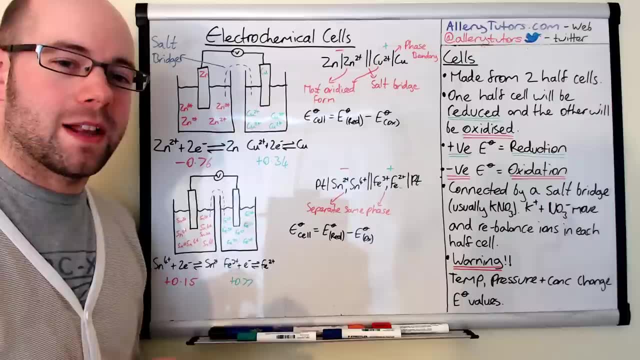 Hi there, my name is Chris Harris and I'm from AllergyTutorscom, and welcome to this video on electrochemical cells. So in this video, we're going to look at what an electrochemical cell is, we're going to calculate the E0 of a cell as well, and we're also going to look at 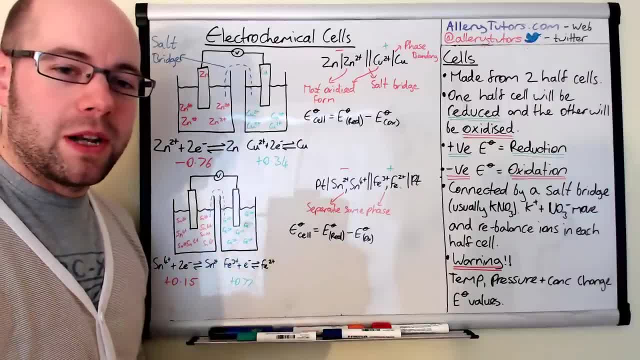 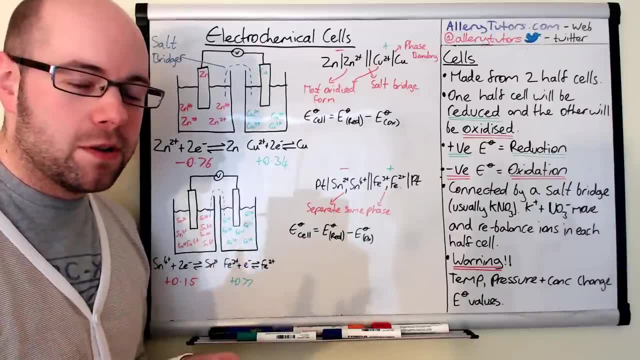 cell representations as well. So we're going to start by looking at how we can construct electrochemical cells, and they're basically made up from two half cells. If you don't know what a half cell is, I have done a video on half cells, so just click on the link below and you can have a.